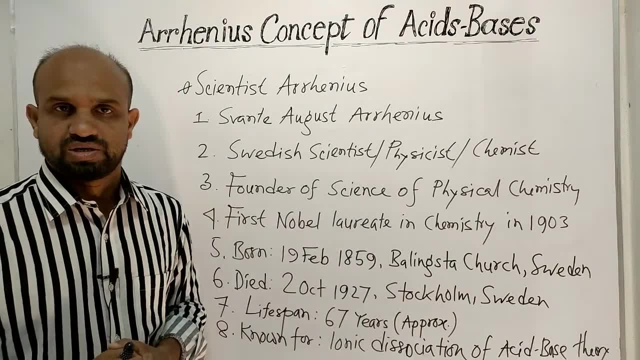 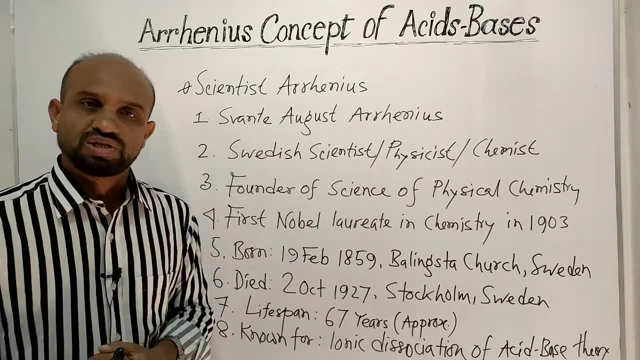 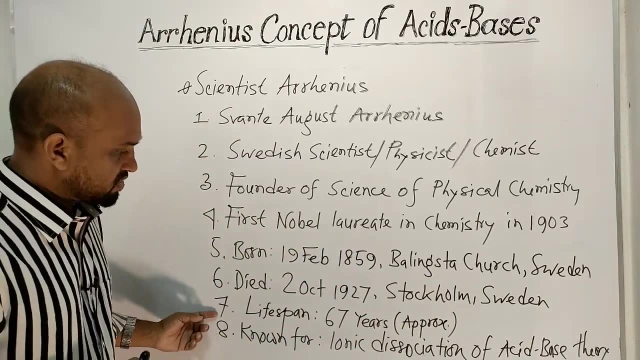 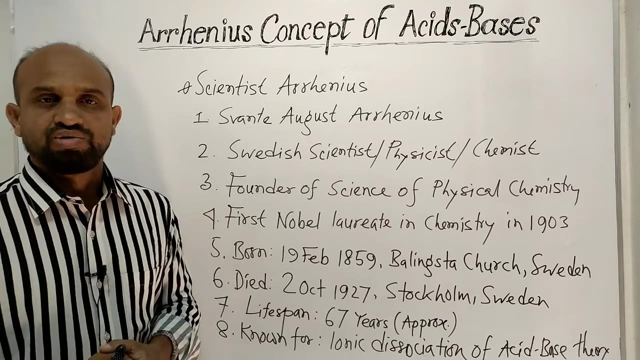 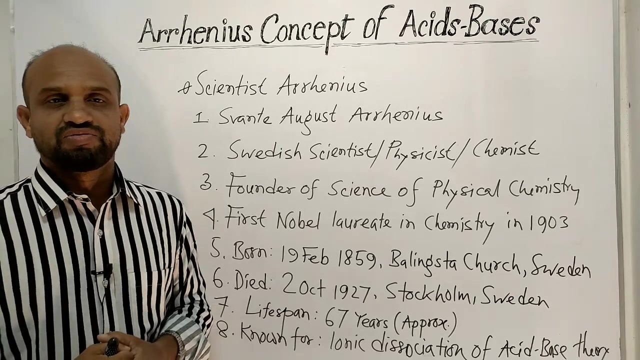 In Bellingenstra church of Sweden. He was died on 2nd October in 1927 in Stockholm of Sweden. Life span was around 67 years. He was known for ionic dissociation of acid base theory. This is most famous topic for short biography of scientist Arrhenius. Let's see next point. 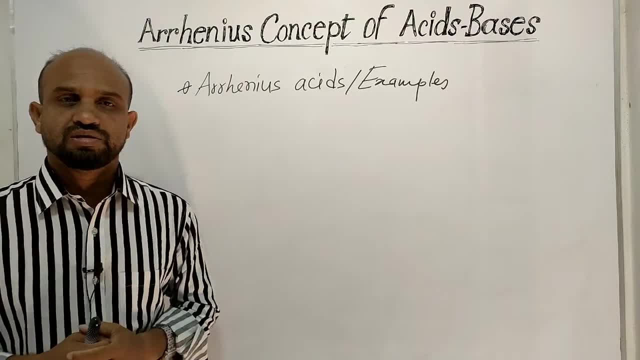 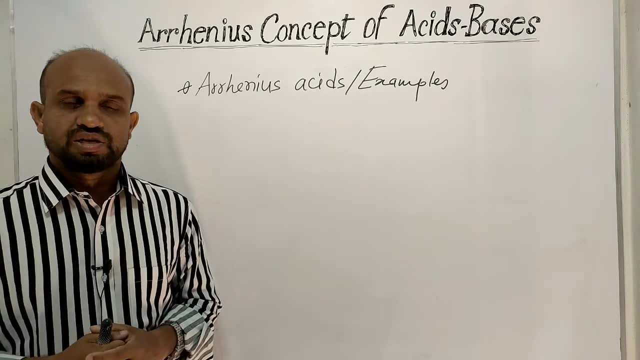 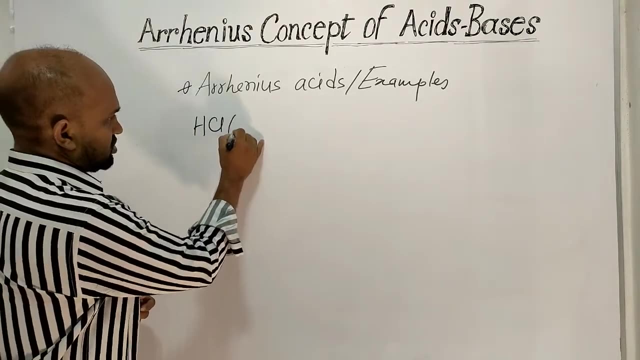 Now the point is Arrhenius acids and examples. let's see some examples and then definition of acids according to Arrhenius theory, windows In hydrogen chloride oxygen is in gaseous state. 賽 김정ensen, Please consider if you want to understand the concept because you used to use downgain acid withùng home, و живaki professor suggests to know how to use it in gasic state or for many processes except the study itself. regard this facility to follow the concept of arhienia acids in a concise sentence and do research. you want to know much more about it. 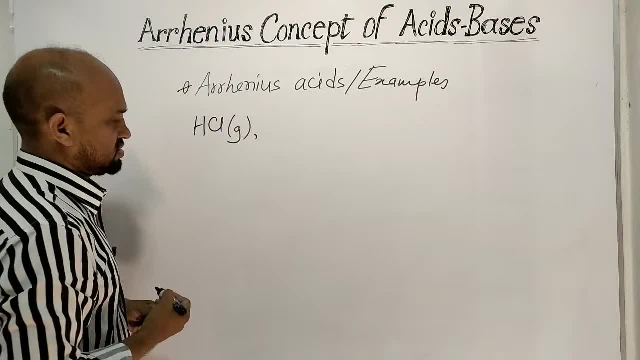 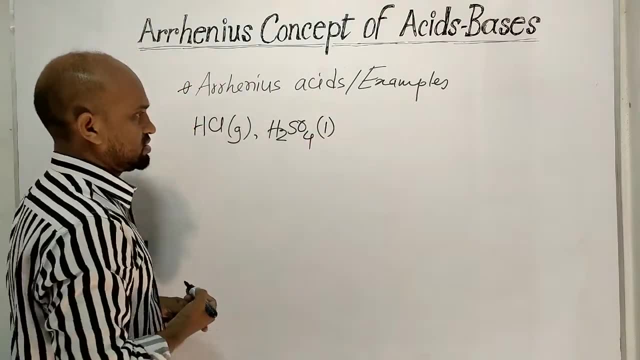 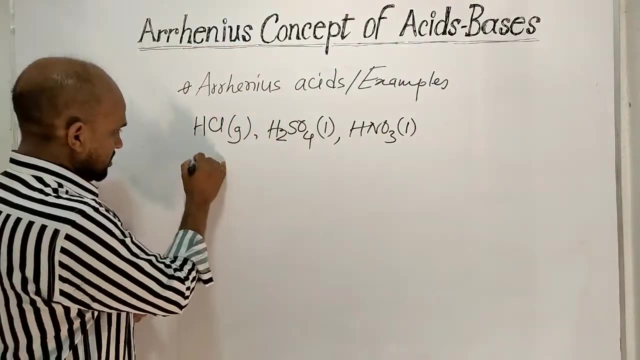 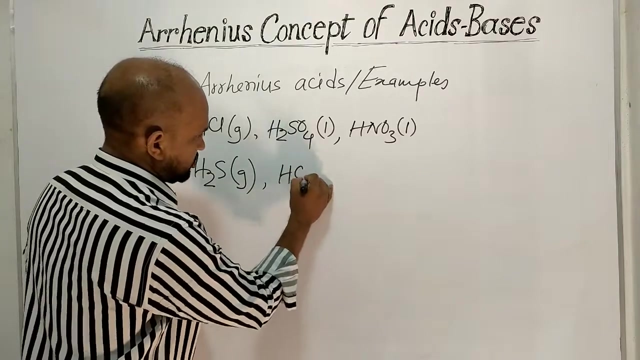 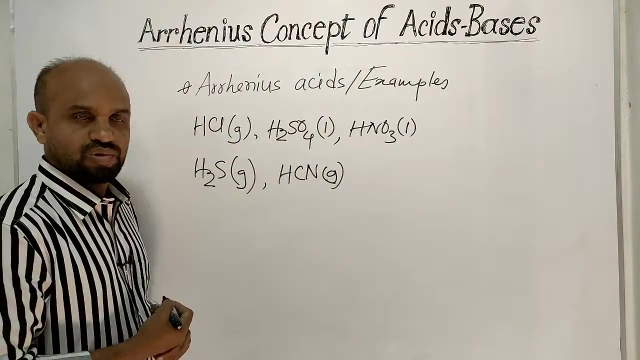 gaseous state. this is Araniac acid, Sulfuric acid, which is liquid in state. Nitric acid, which is liquid in state. Hydrogen sulfide, which is gaseous in state. Hydrogen cyanide, gaseous in state at normal condition. 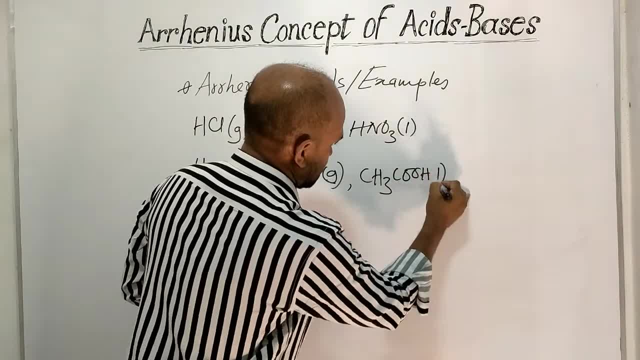 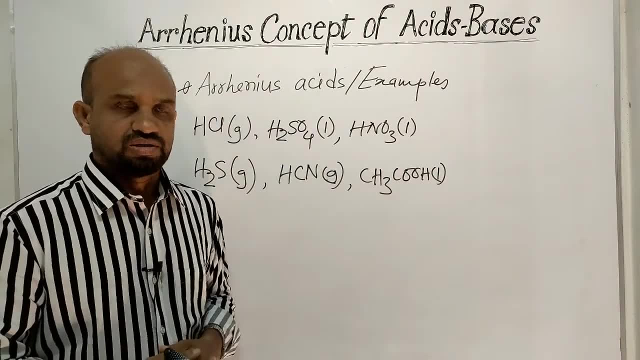 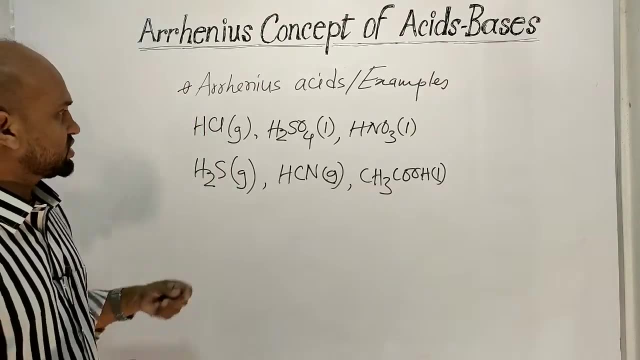 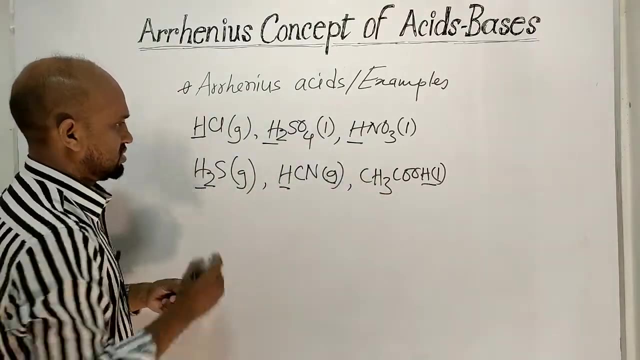 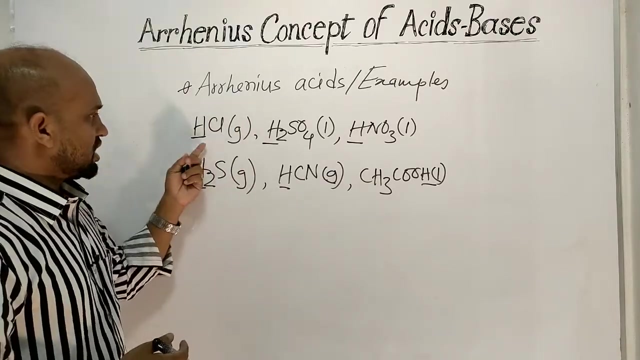 Acetic acid. the state of acetic acid is liquid at normal condition. these are the examples of Araniac acid. here one thing is observed: that all the compounds have hydrogen hydrogen. so definition of Araniac acid is the hydrogen containing compounds that give protons in. 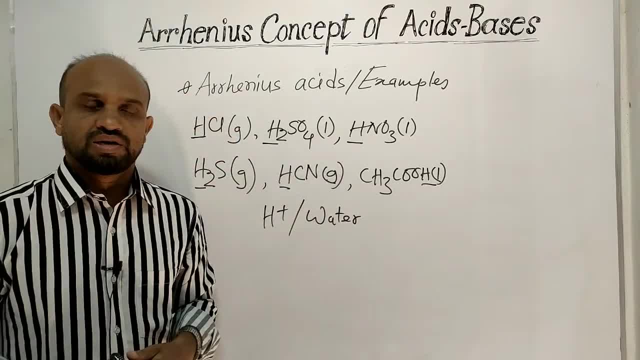 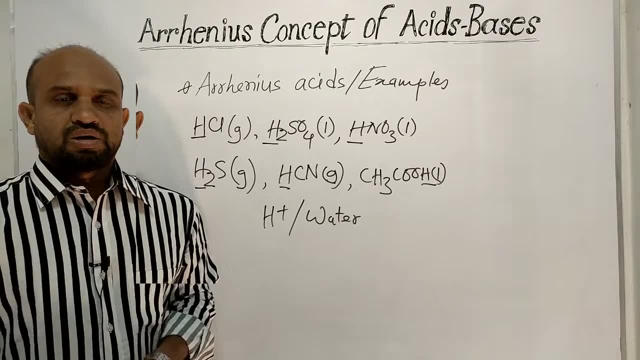 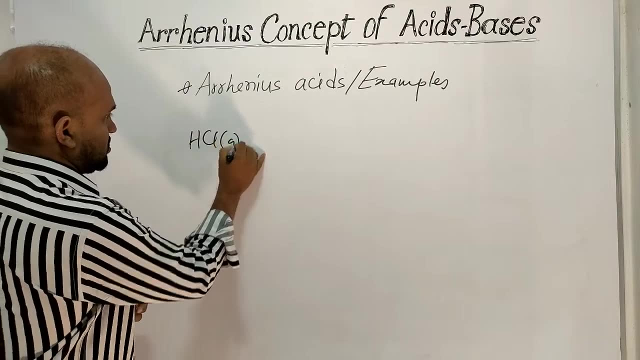 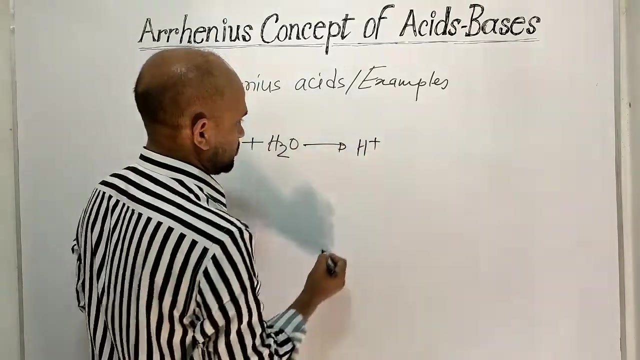 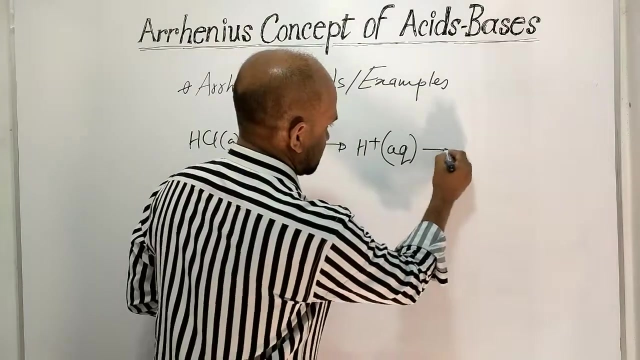 water are called Araniac acid. now let's see how these compounds produce protons in water, hydrogen chloride, which is gaseous in state. when it is dissolved in water, then proton is produced which is surrounded by aqua. that means water. at the same time. 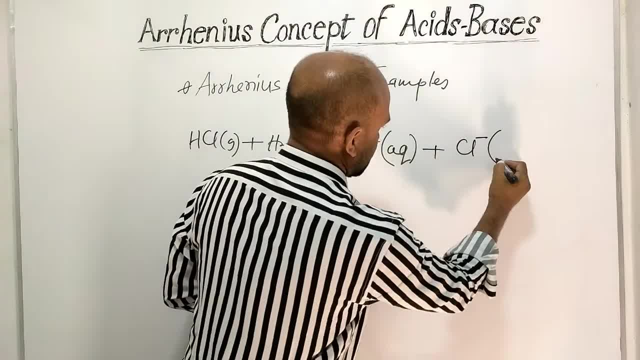 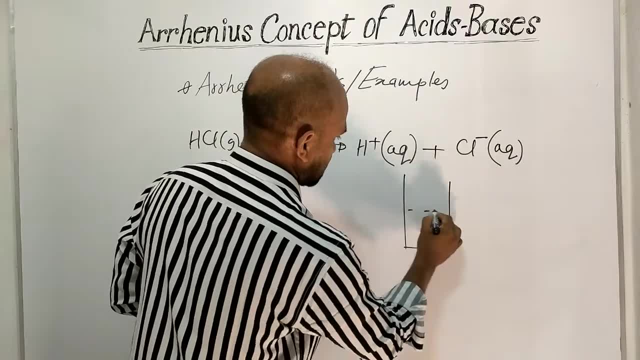 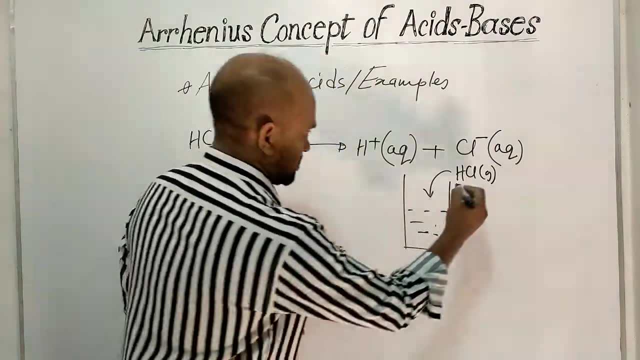 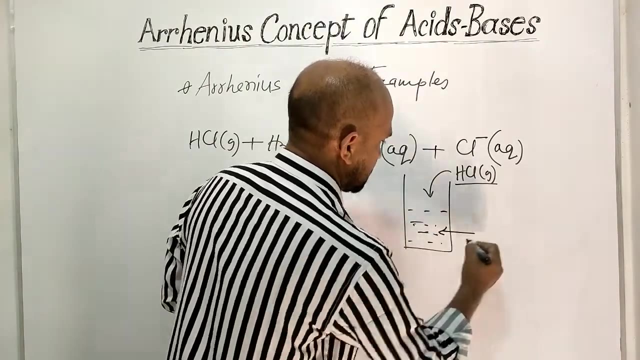 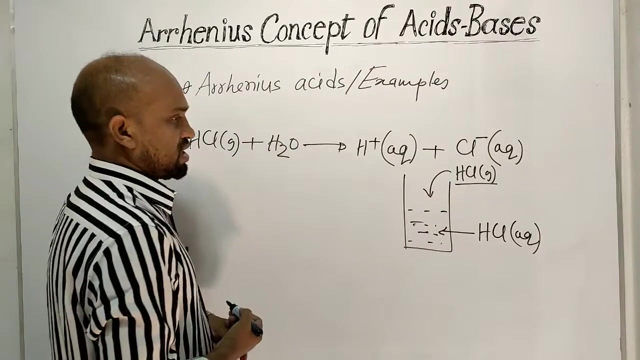 chloride ion is formed. this is also surrounded by aqua. that means water here, when suppose this is water? and hydrogen chloride gas is dissolved here. this is hydrogen chloride. and after dissolving hydrogen chloride, the solution obtained is symbolized by acl aqueous, that means hydrochloric. 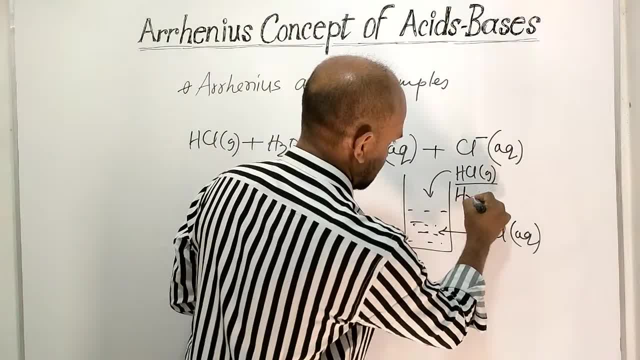 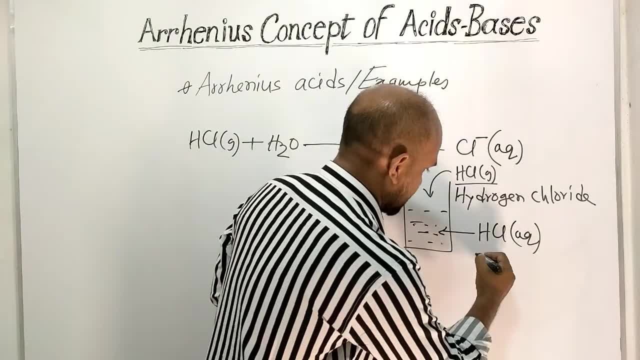 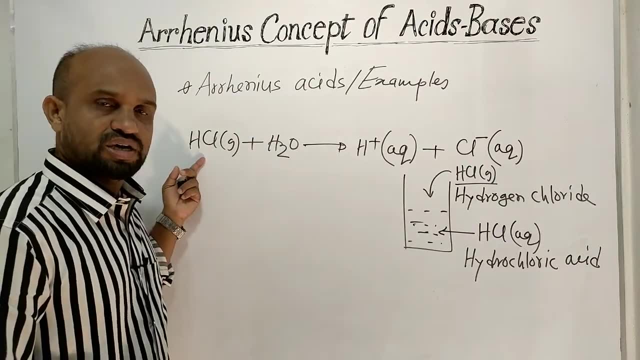 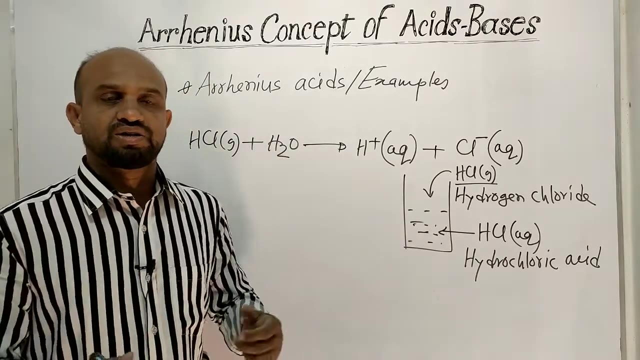 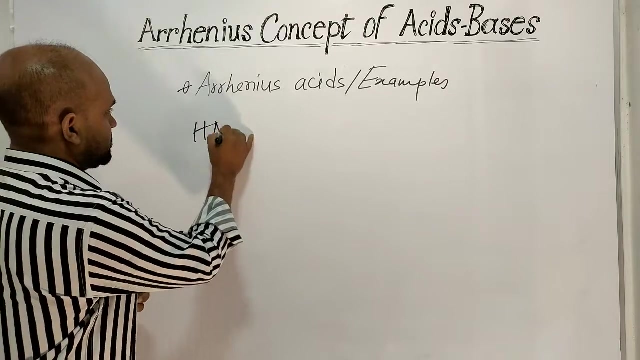 acid. this is hydrogen chloride, and the acetic form of hydrogen chloride is hydrochloric acid. so this is the way in which hydrogen chloride gas produces proton in water. so hydrogen chloride gas is a kind of Araniac acid. now the acid is nitric acid, HNO3. 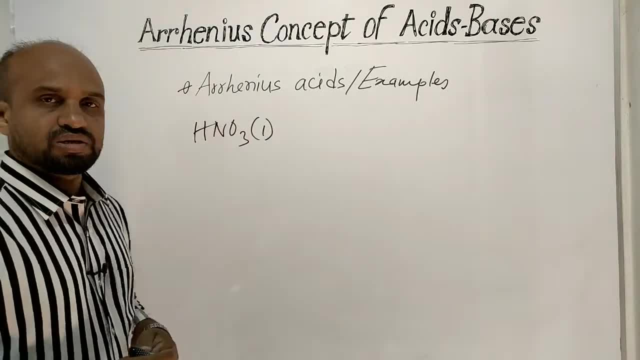 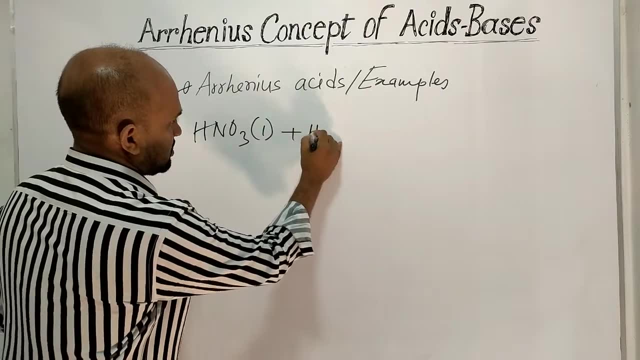 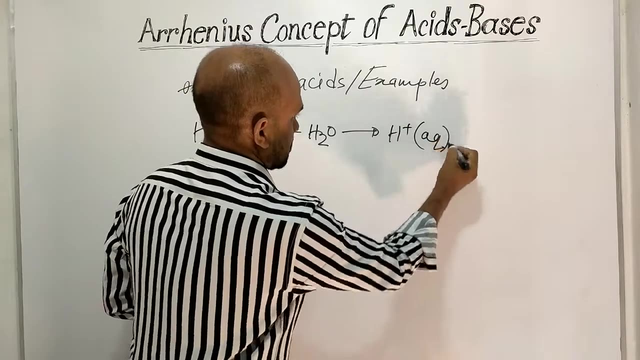 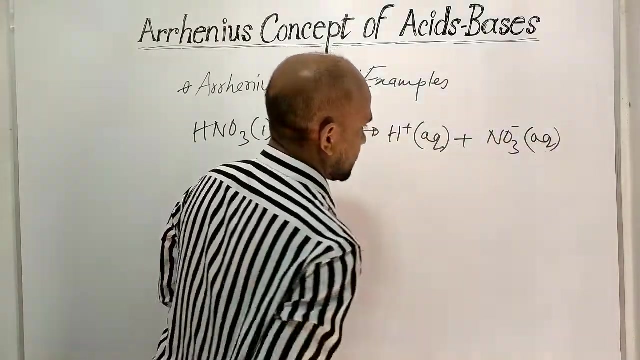 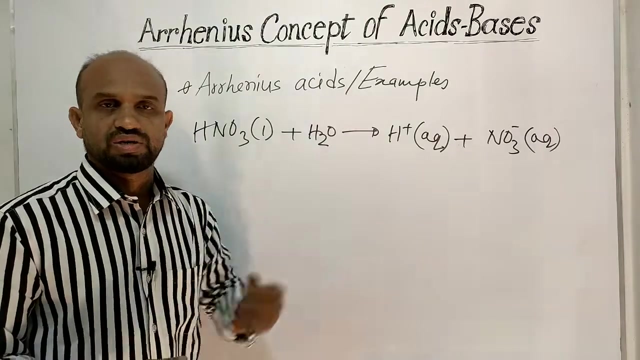 which is liquid state at normal condition. when this nitric acid is added to water, then proton is formed, surrounded by water, and nitrate ion is formed, which is surrounded by water as well, since this compound produces proton in water. so nitric acid is a kind of Araniac acid. 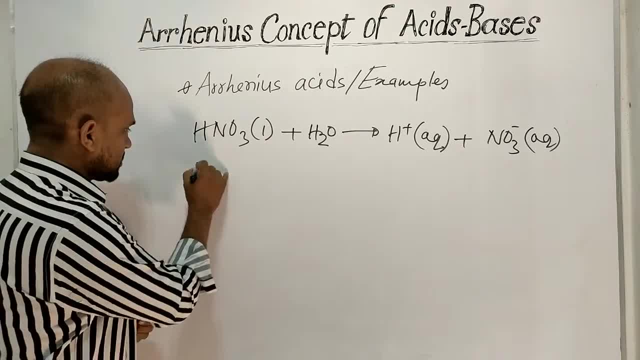 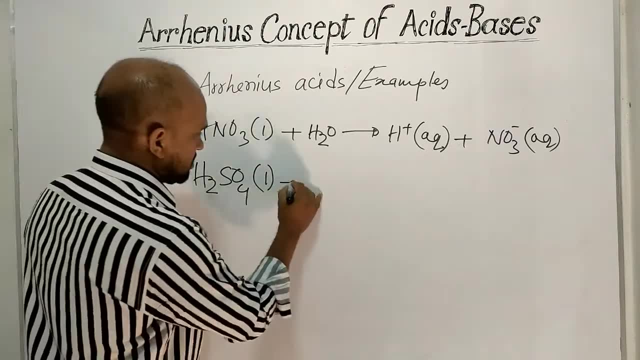 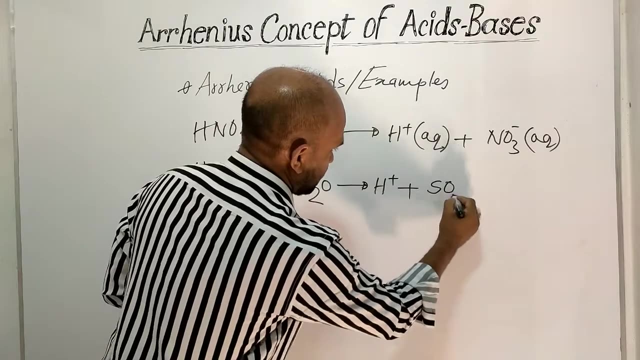 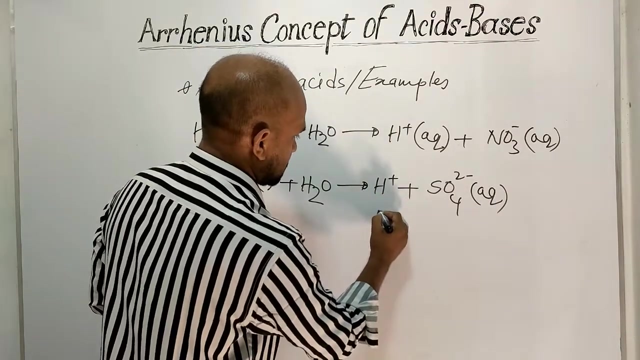 now let's see a sulfuric acid, H2SO4, which is liquid at normal condition. when it is added to water, then proton is formed. at the same time, sulphate ion is formed, which is surrounded by water. this proton is surrounded by water as well. sometimes it is. 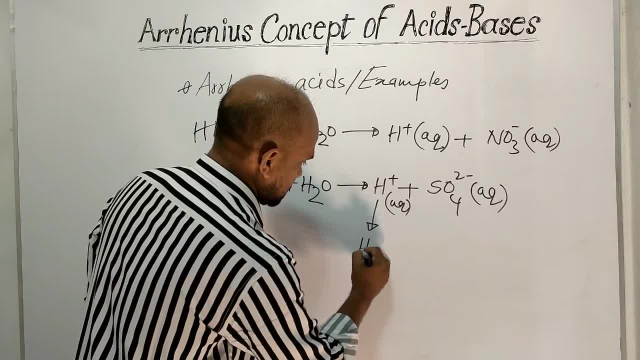 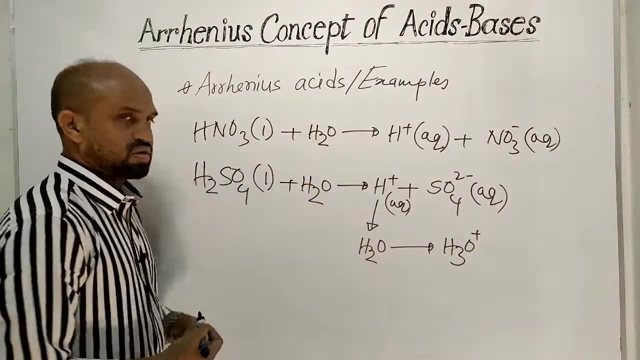 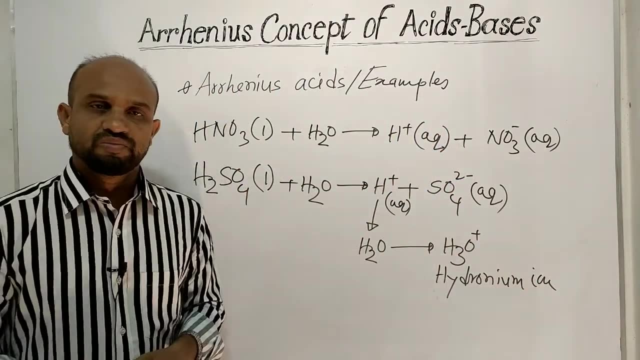 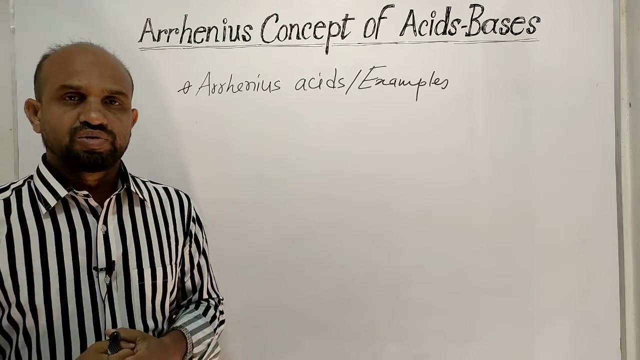 showed in this way. that is, this proton is added to water molecule and this ion is formed, which is called hydronium ion. so sulfuric acid is a kind of Araniac acid. let's see some more acids now. the compound is hydrogen sulphate. 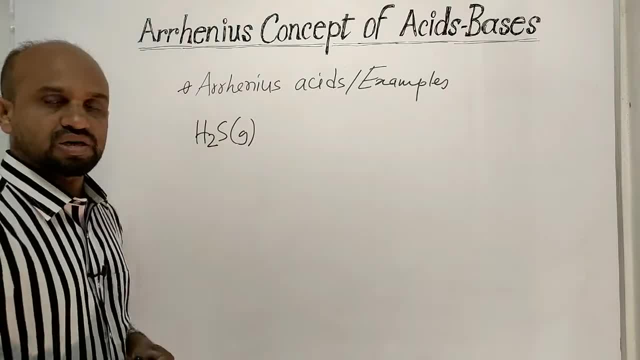 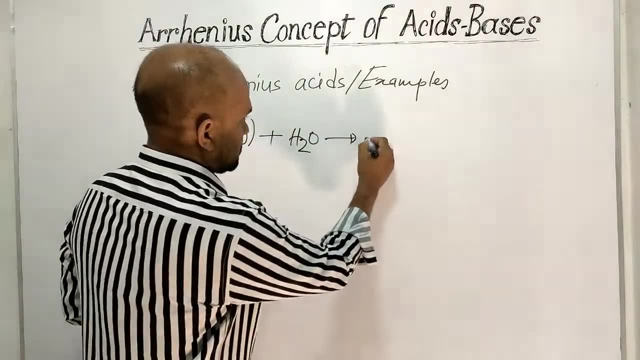 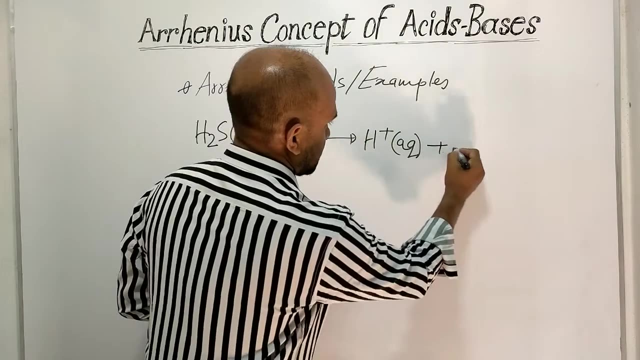 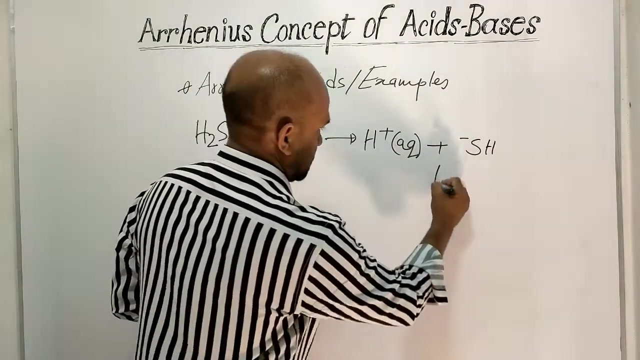 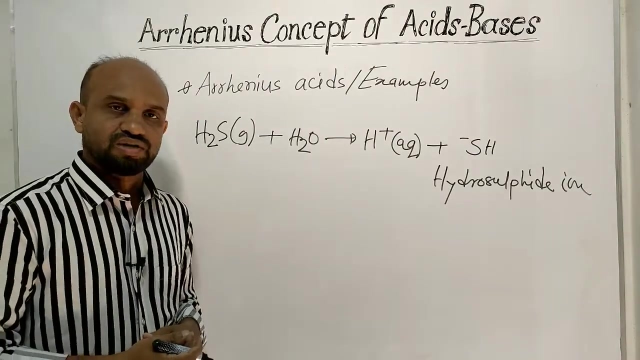 which is gaseous at normal condition. when it is dissolved in water, then it yields proton, which is surrounded by water, and another ion is formed, that is hydrosulphide ion. hydrosulphide ion is formed. this is hydrogen sulphate. 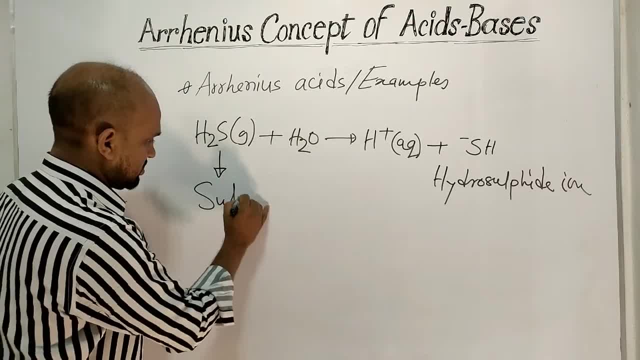 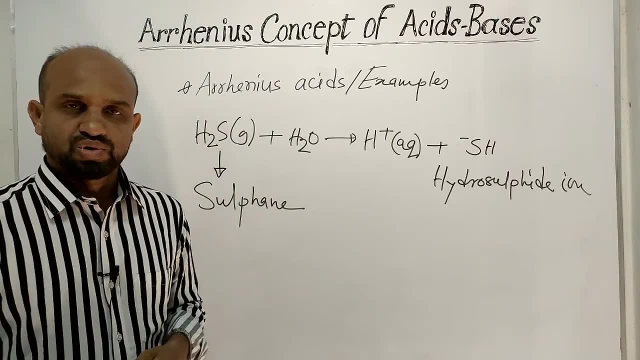 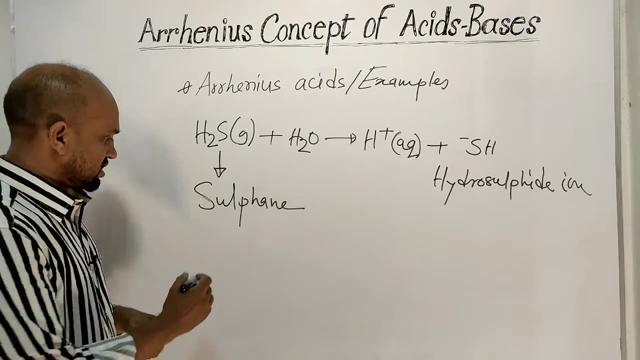 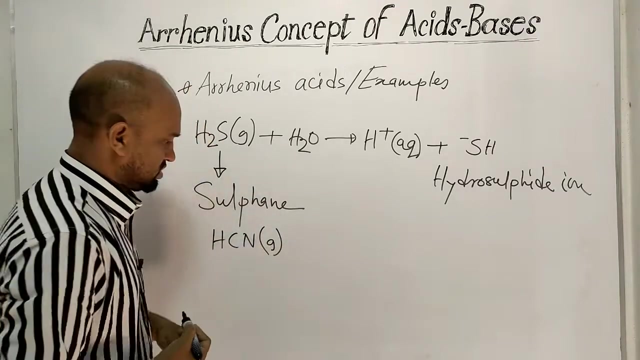 it's another name is sulfane, so hydrogen sulphate can produce protons in water, so hydrogen sulphate is a kind of Araniac acid. let's see another acid, that is hydrogen cyanide, which is gaseous in state and when it is dissolved. 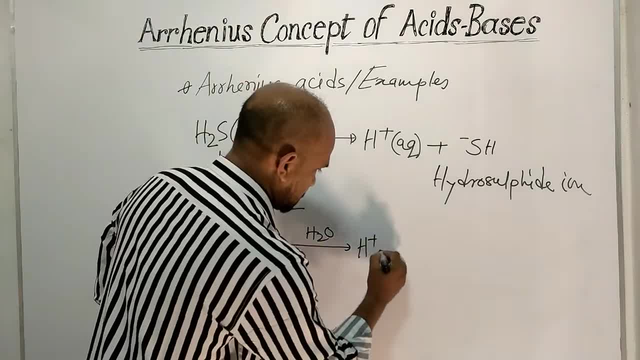 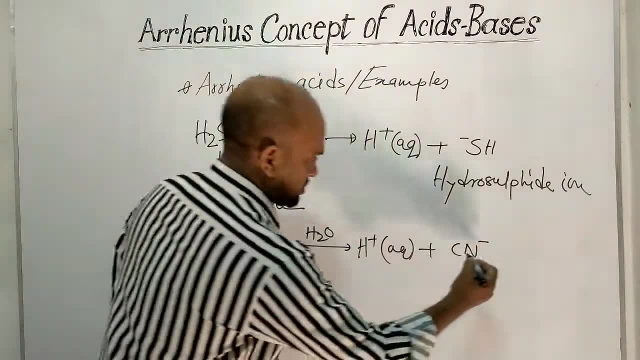 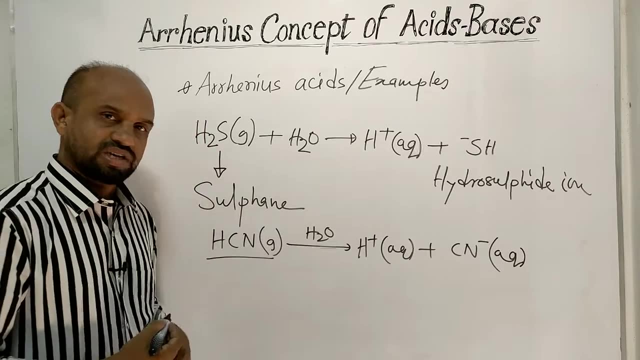 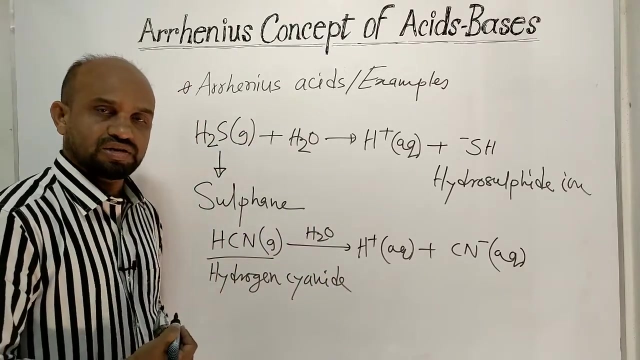 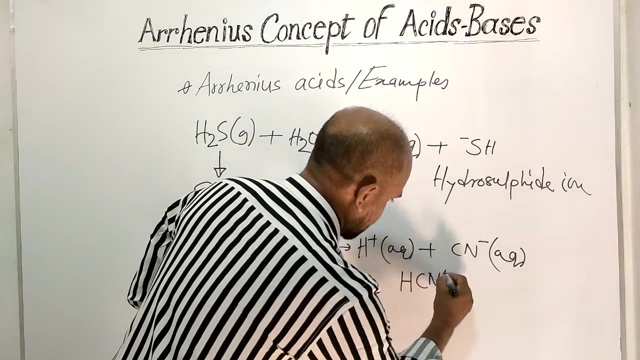 in water, then proton is formed and cyanide ion is produced, which is surrounded by water. now its name is hydrogen cyanide. but when this hydrogen cyanide gas is dissolved in water, then a solution is obtained. this is symbolized by hydrogen cyanide, now its name is: 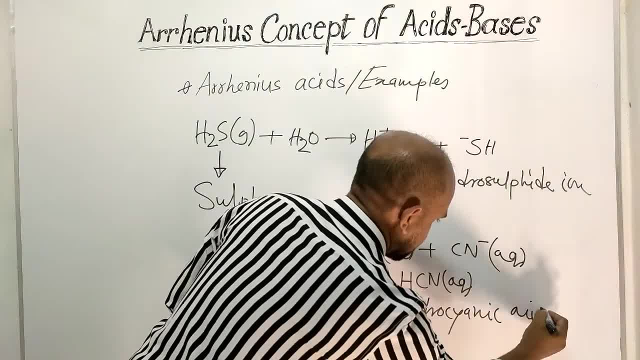 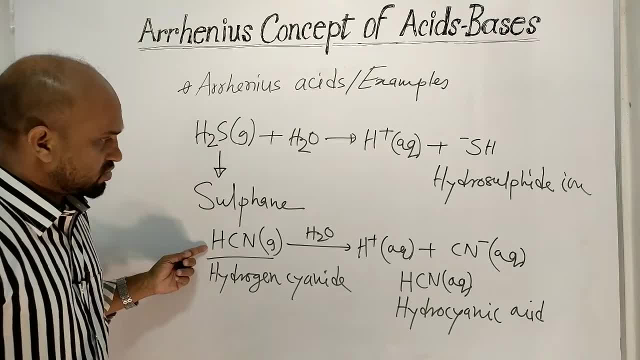 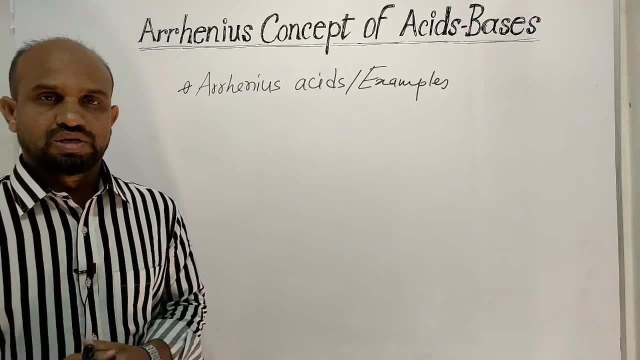 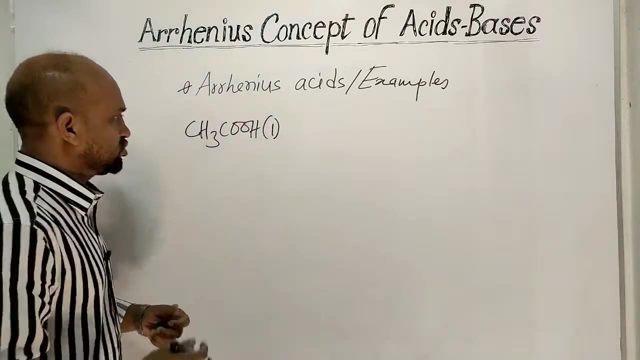 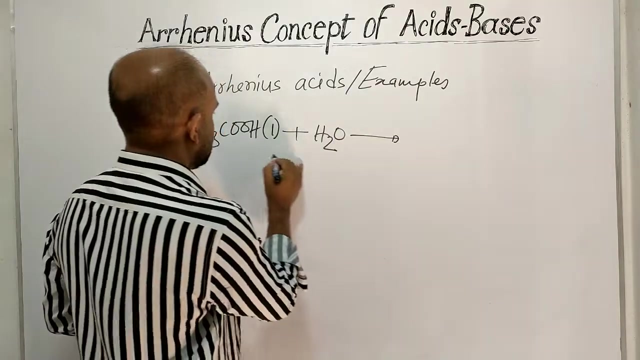 hydrocyanic acid. so hydrogen cyanide is a kind of Araniac acid, because it can produce proton in water. let's see another acid now. the acid is acetic acid, which is liquid at normal condition. when it is dissolved in water, then this hydrogen is released. 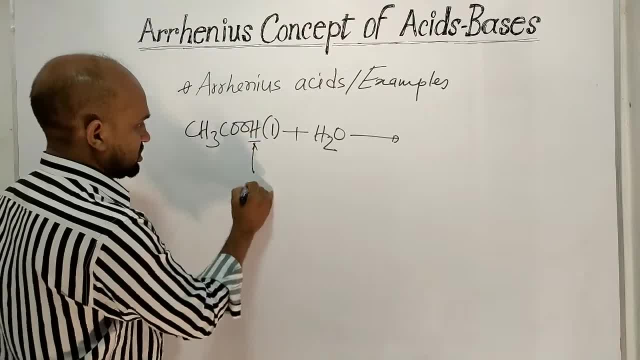 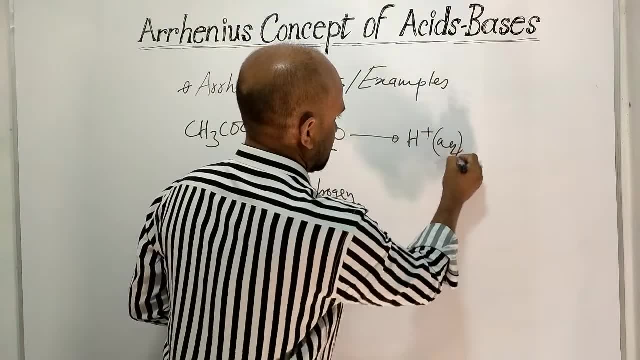 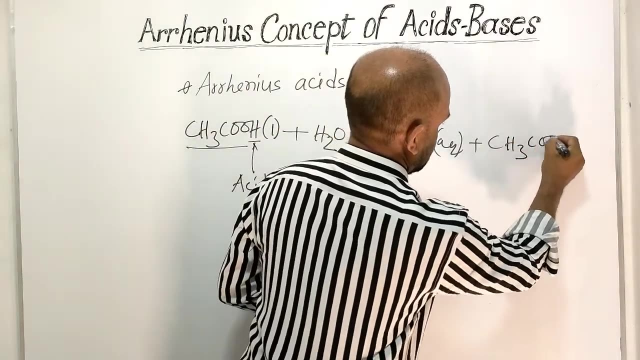 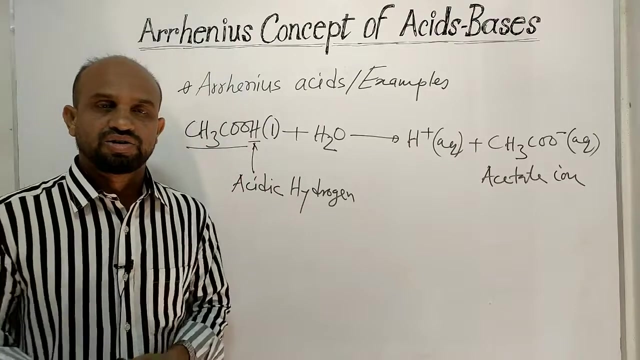 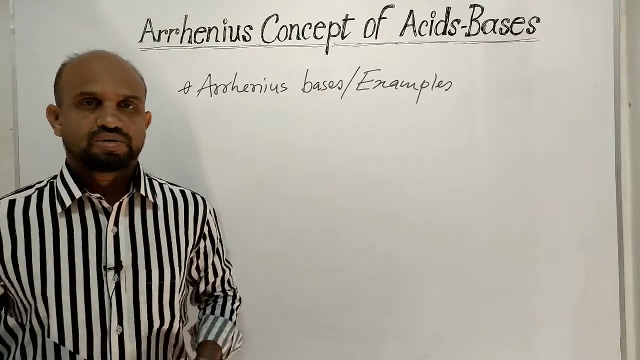 as proton, which is called acetic hydrogen. it is released as proton and another anion is formed, that is acetate ion. so acetic acid is a kind of Araniac acid, because it can produce proton in water. let's see the next point now. the point is: 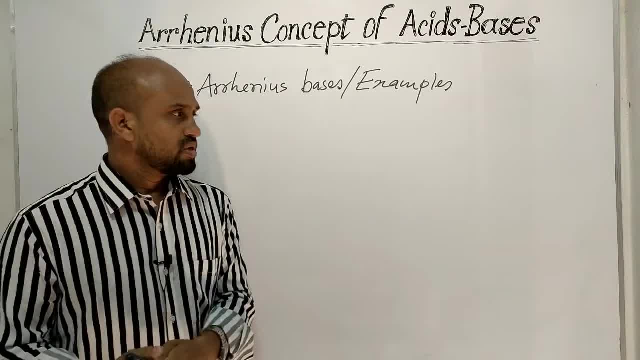 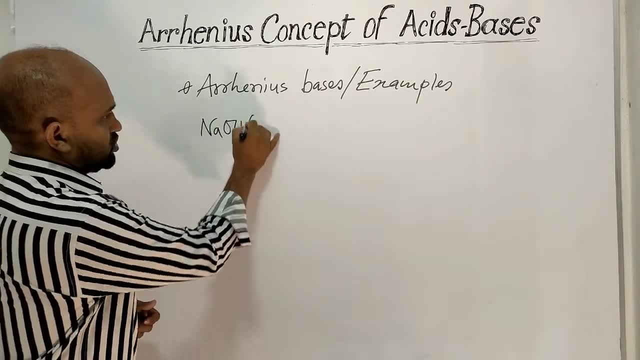 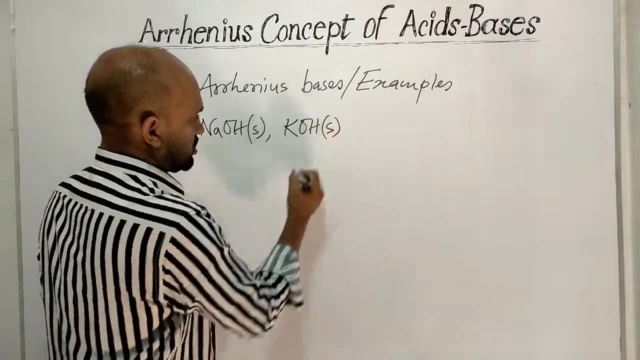 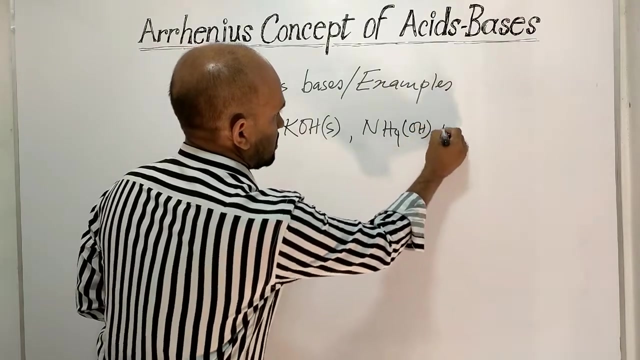 Araniac bases with some examples. let's see some examples of Araniac bases. that is, sodium hydroxide, which is solid at normal condition. potassium hydroxide, solid at normal condition. ammonium hydroxide, which is liquid at normal condition. so this compounds are 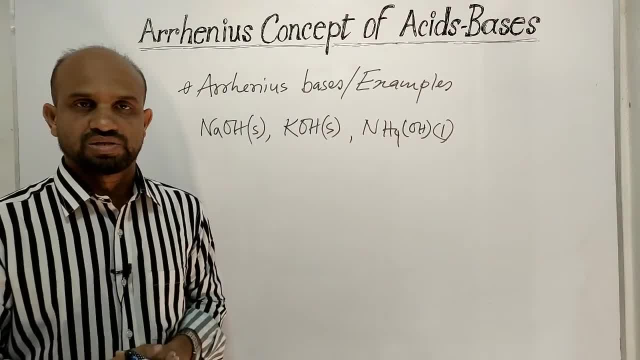 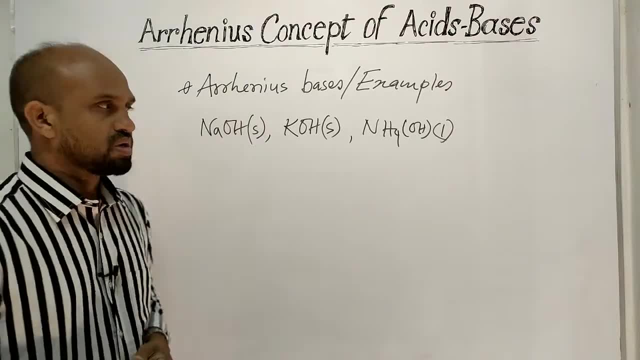 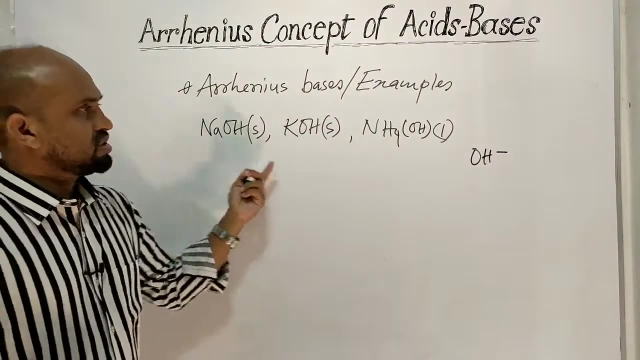 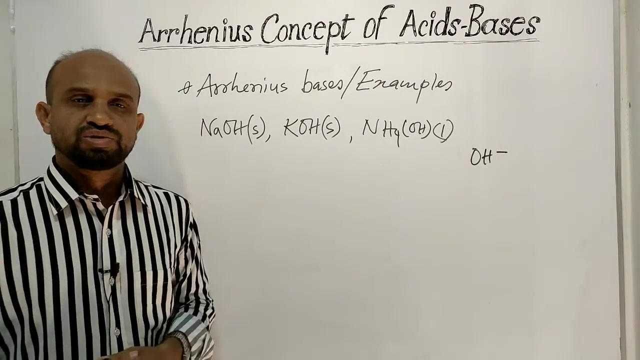 Araniac bases. one thing is observed here: that all the compounds have hydroxide ion. this is hydroxide ion, so the definition is: the compounds are hydroxide. compounds that can produce hydroxide ion in water are called Araniac bases. let's see. 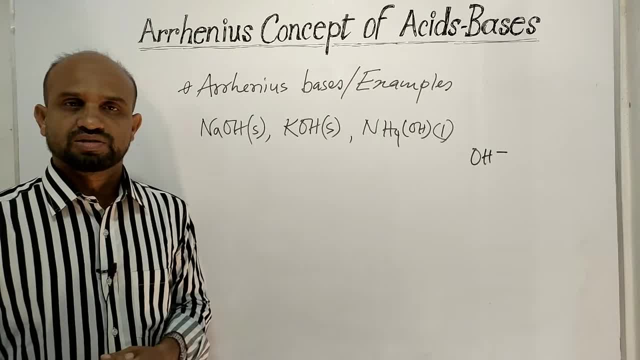 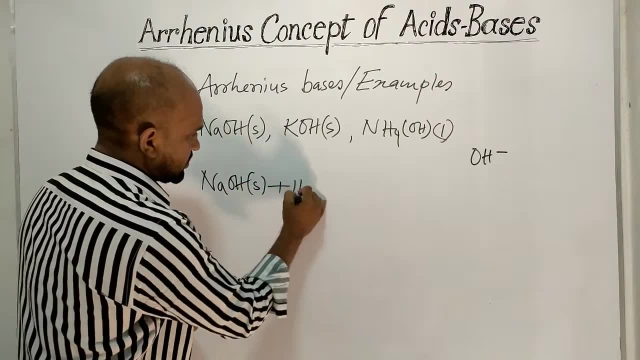 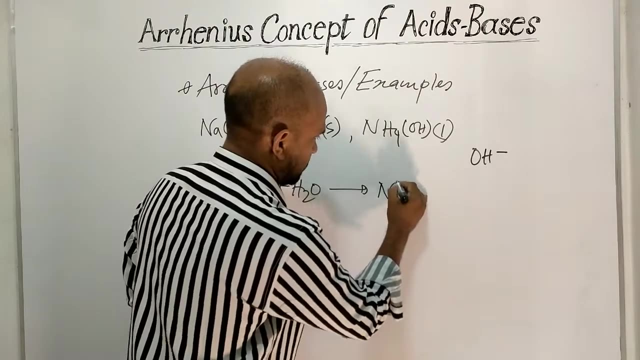 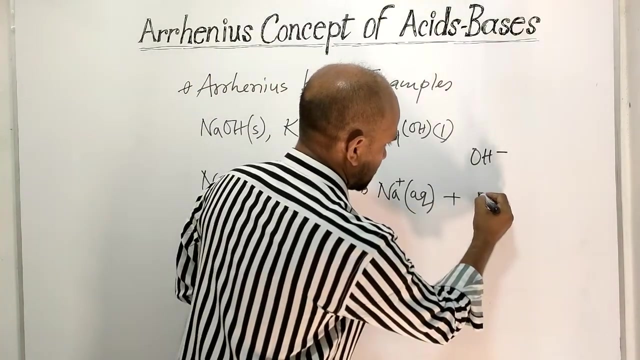 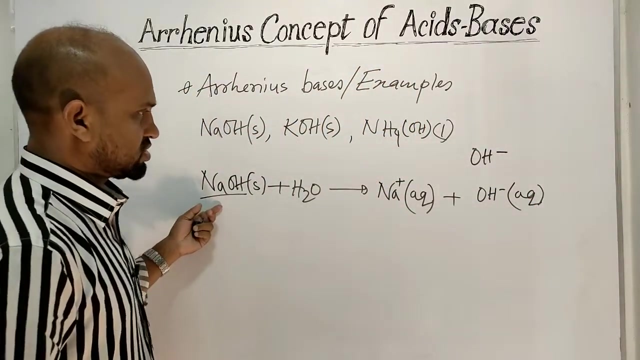 how this compounds produce hydroxide ion in water. when sodium hydroxide is dissolved in water, then it ionizes and sodium cation is formed, which is surrounded by water. at the same time, hydroxide ion is formed, which is surrounded by water. so sodium hydroxide 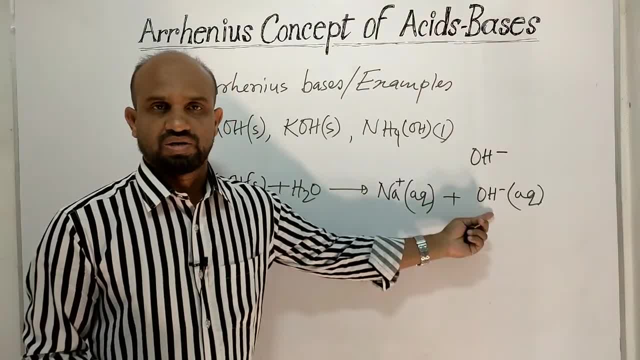 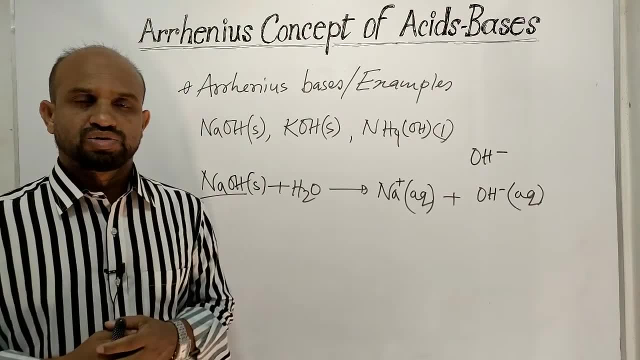 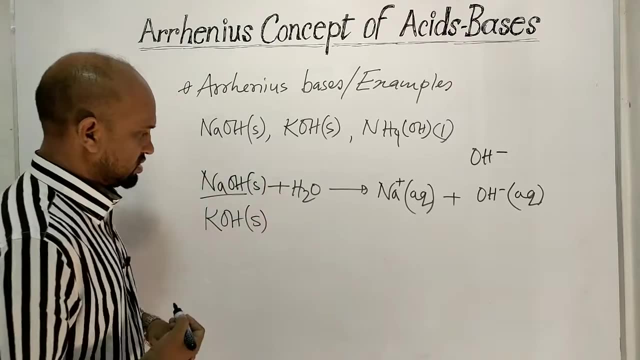 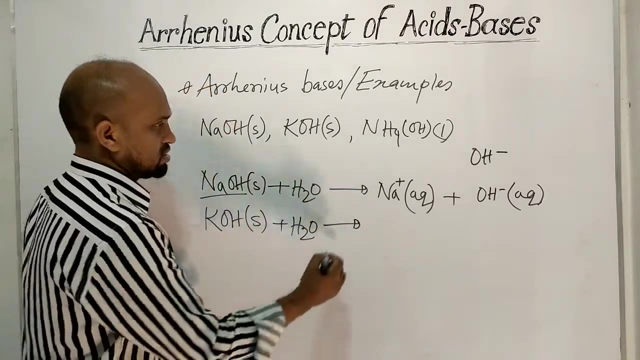 can produce hydroxide ion in water. so sodium hydroxide is a kind of Araniac base. let's see about potassium hydroxide: potassium hydroxide, which is solid at normal condition. when it is dissolved in water, then potassium ion is formed, which is 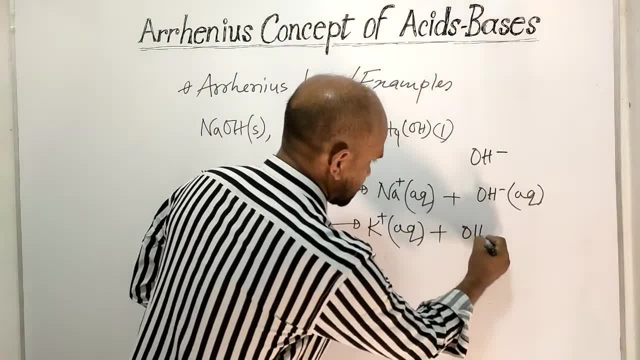 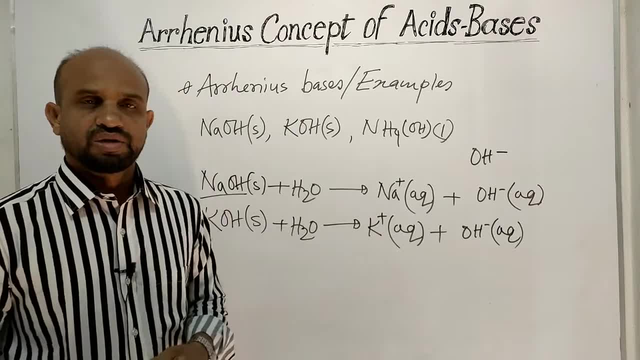 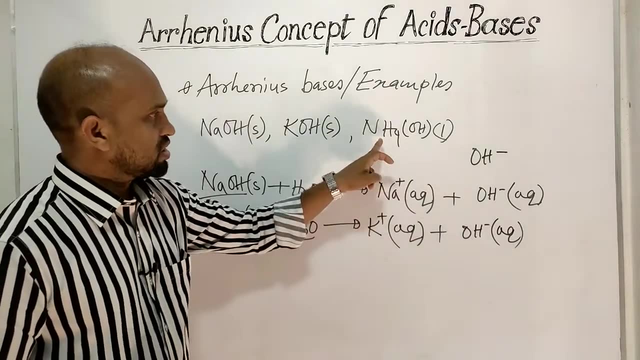 surrounded by water. at the same time, hydroxide ion is formed, which is surrounded by water. so potassium hydroxide is a kind of Araniac base, because it can produce hydroxide ion in water. now let's see about ammonium hydroxide.